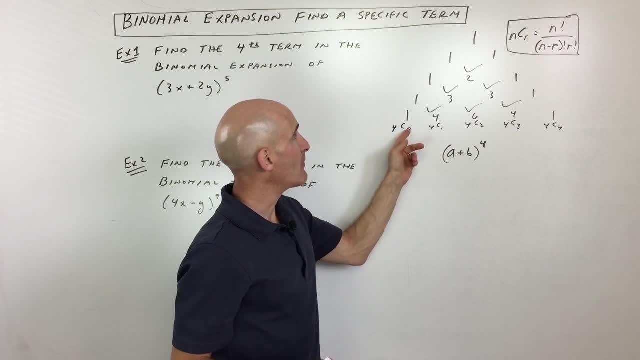 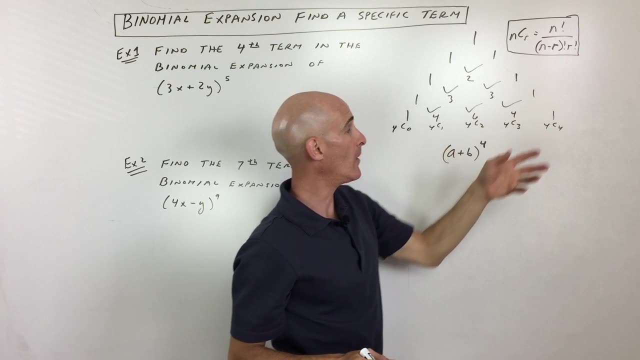 from there. okay. Now, when you work with combinations, we use this formula: here, ncr equals n factorial over n minus r factorial, r factorial. So I'll give you an example like, say, if we wanted to expand out a plus b to the fourth power, Well, what we can do is we can. 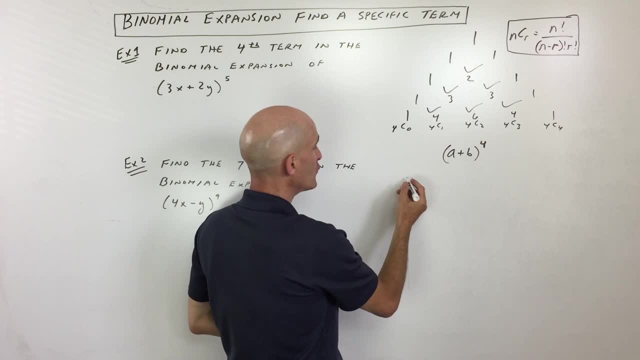 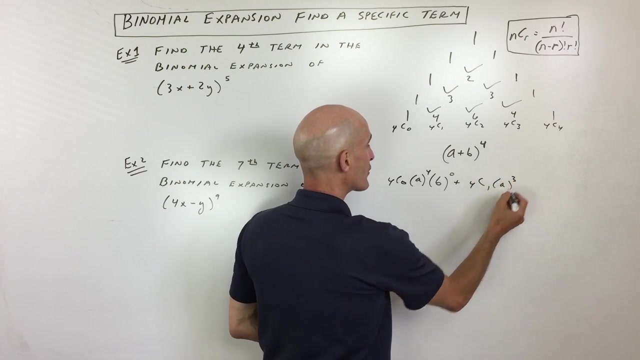 say: well, we're on the fourth row, so we're going to do four, choose zero. and then what you do is first term, a to the fourth power, and you take the second term, b to the zeroth power. Now, when you go to the next term, you're going to do four, choose one. This is going to be a to the third. 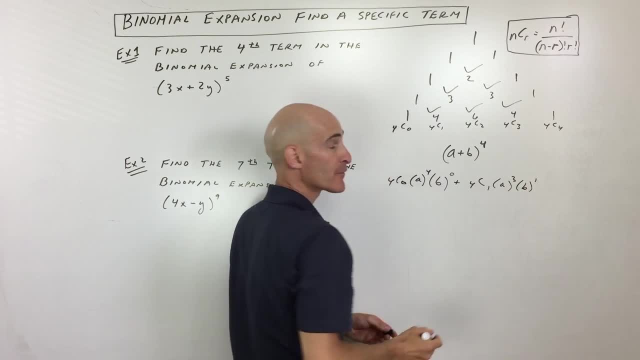 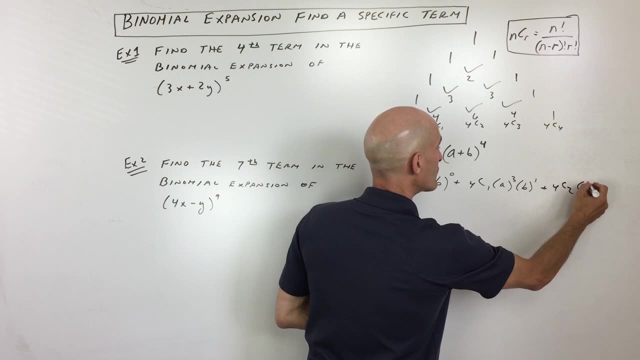 power. See, I'm going down, but the second term is going to be b to the first power. Notice I'm going in ascending order or up. So if we continue on, you can see: four choose two. Now we're going to be at a squared, b squared and I'll just carry that over here. four choose three: a to the first. 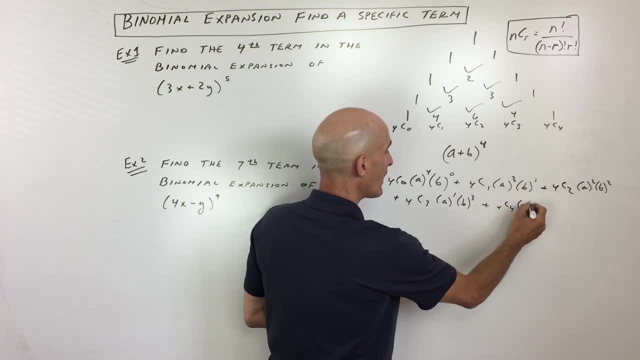 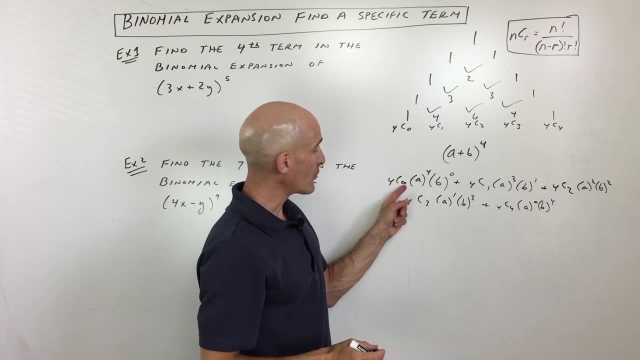 b to the third And lastly, four. choose four: a to the zero and b to the fourth. Now one thing I want you to notice real quick is that see how this second number here, this r value, see this is zero and this: 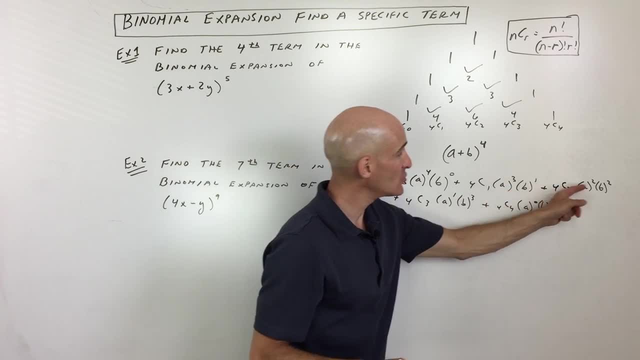 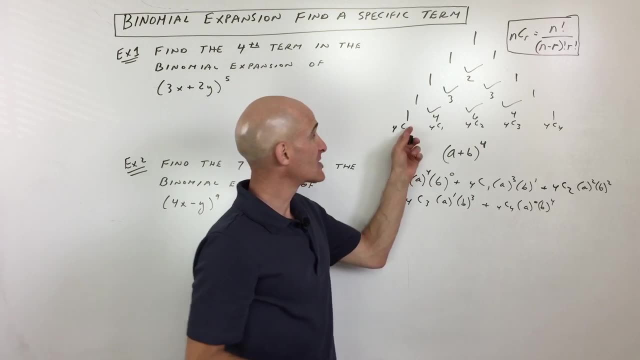 second term's power. see how that's zero: One, one, two, two. see the pattern. Also, notice that when you add these exponents, four plus zero is equal to four. That's the power, that's the row that we're working with right. So if we recognize that pattern, we can use that to zero in on a. 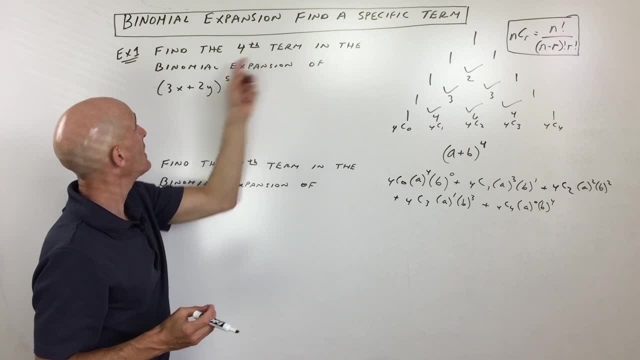 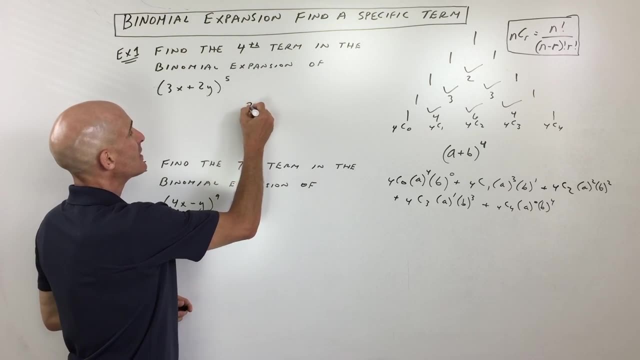 specific term. So for example, here see how it says: find the fourth term in the binomial expansion of 3x plus 2y to the fifth. Now follow how I'm going to do this. This makes it a lot easier to do it in this way. So I'm going to take 3x. 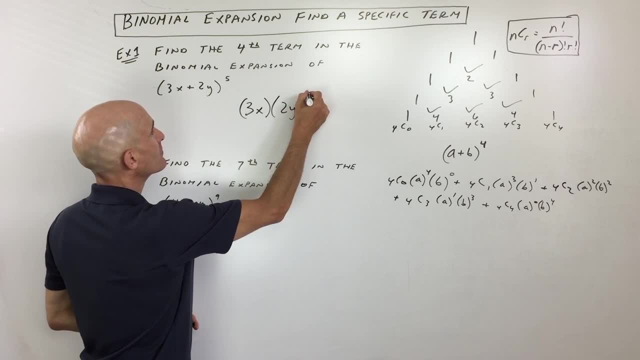 that's the first term. 2y, that's the second term. okay, And then what I'm going to do. the fourth term now notice over here, like if I wanted to find the. let's just say I wanted to. 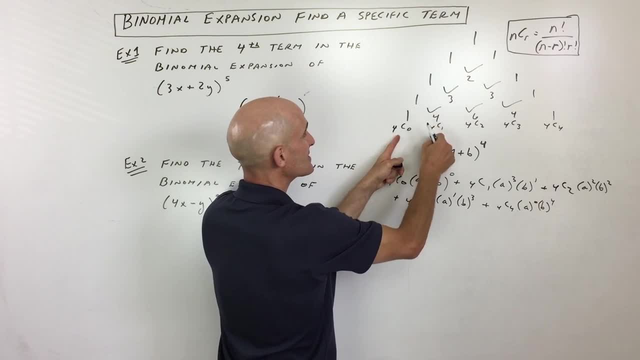 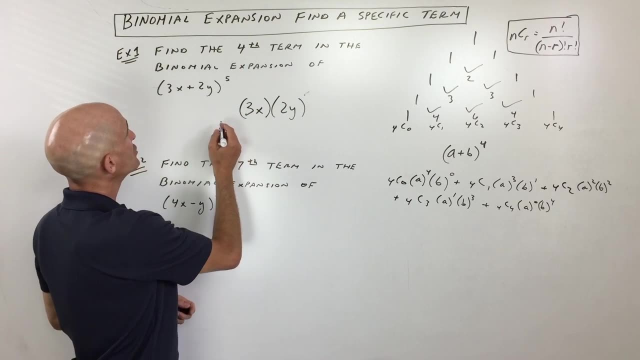 find the second term. this is the first term. this is the second term, but see how this is just four, choose one. That's because we're starting at zero, So when I go over here to the fourth term, I'm going to be at three, and this is the fifth row. so this is going to be five, choose three. Okay. 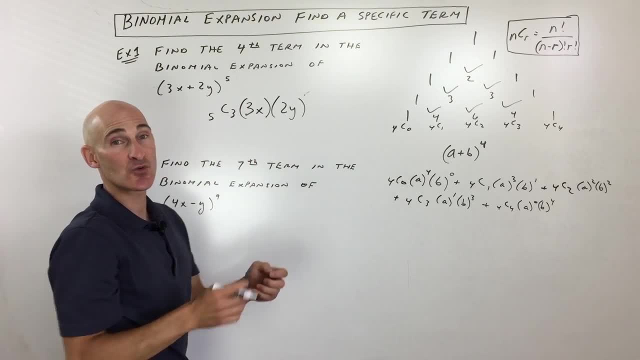 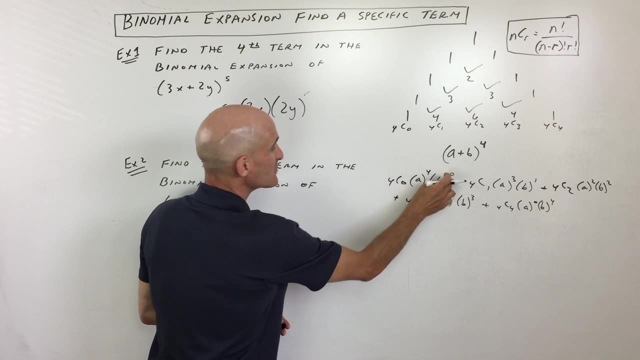 so if I went down to this fifth row, the fourth term would actually be five, choose three, because you're going zero, one, two, three. right Now. remember the pattern, how I said that this r value and this second term's power. see how they always match. So if this is a three here, this is going. 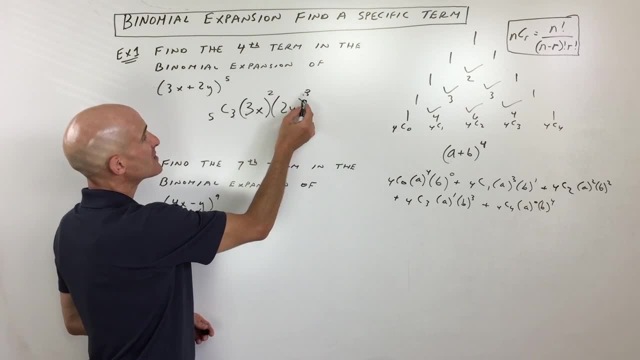 to be a three here. this is going to be a two, because three plus two adds up to five. That's the power, okay, So now all we have to do is simplify this down. So five, choose three. I'm going to be. 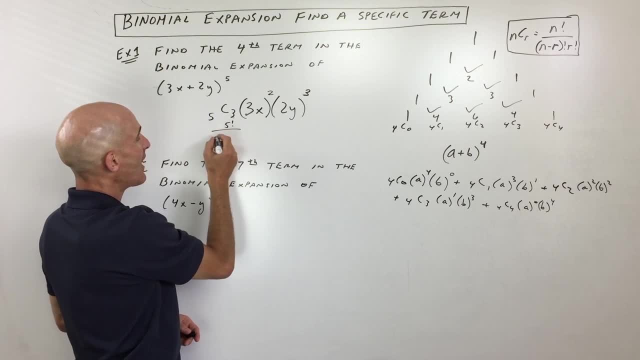 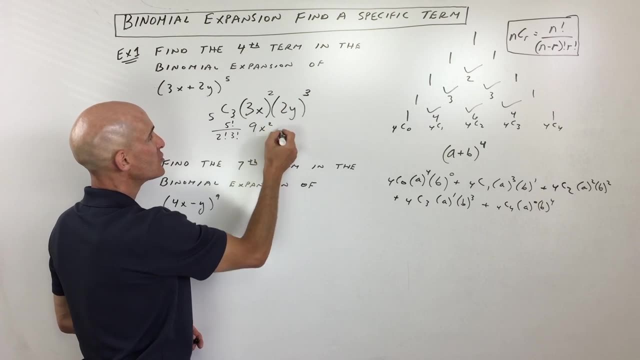 using the elimination formula here. so this is five factorial over five minus three, which is two factorial times three factorial, and this is three squared, which is nine. x squared two cubed is two times two times two, which is eight. and now, if I simplify this, five factorial is what It's five. 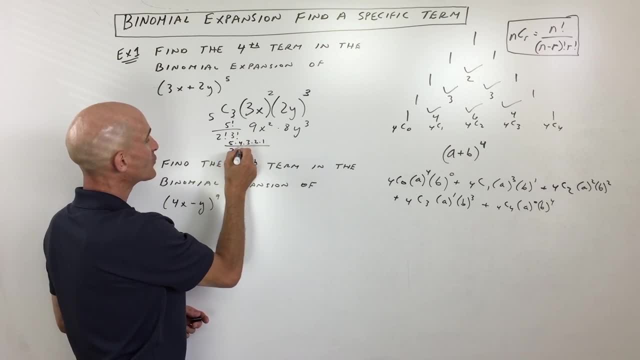 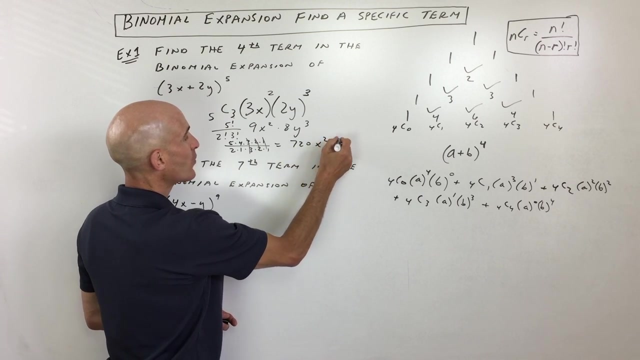 times four times three times two times one, all over two. factorial, that's two times one times three. factorial, that's three times two times one. but you can see those are canceling. This is 20, so I get 10 times nine times eight is 72, so I get 720 x squared y cubed. They want that particular. 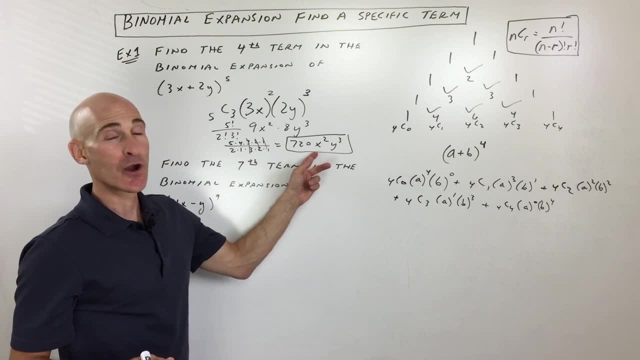 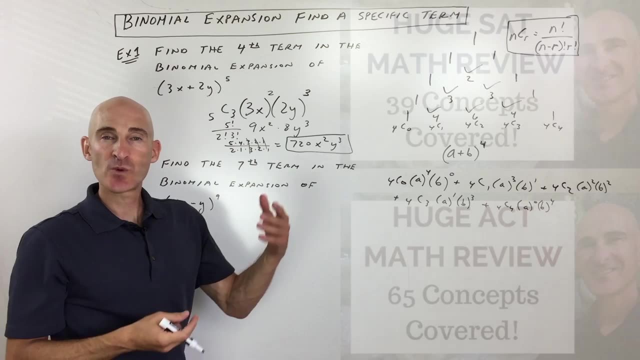 term. they want that whole group, and so that's going to be your answer there. Now we're going to go to the next example, but I know a lot of students right now are preparing for the ACT and the new SAT, so I just wanted to let you know about my two courses. my huge ACT math review video. 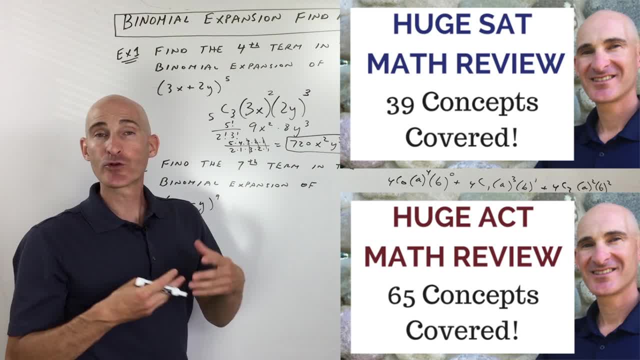 course and my huge SAT math review video course. We go through teaching, we go through formulas, we go through things that you would see on those tests On the math section. we talk about how to recognize them and how to approach those problems. So go over there, check out the link and there's three free. 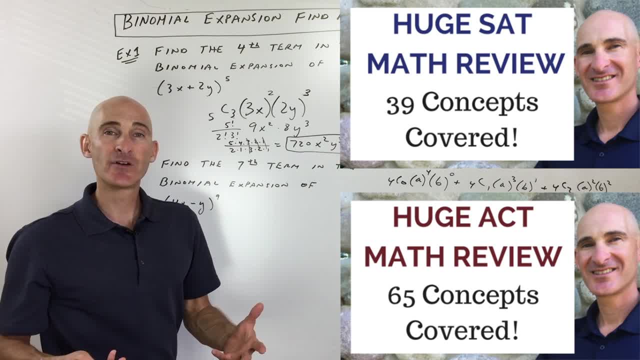 lessons in both those courses. You can take those lessons, get a sense of, you know how the course is laid out and if it's right for you and you'll get benefit right from the start from taking those lessons. and if you want to go further, you can purchase the course and you know, learn more. 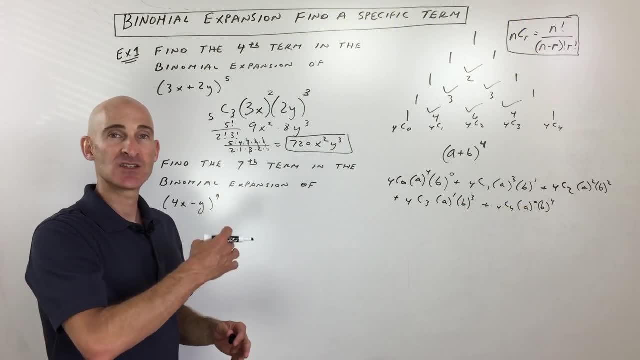 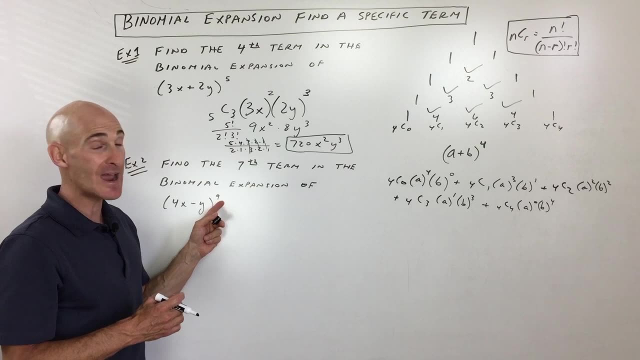 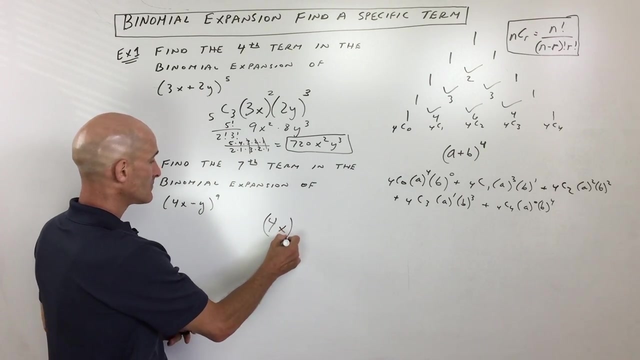 about how to prepare for those two tests. But let's go ahead and jump back into this video, talking about finding a specific term In the binomial expansion of 4x minus y to the ninth power. we want the seventh term here, So, hmm, so what are we going to do? Well, what I'm going to do is I'm going to say 4x negative y. Okay, so those are our two terms. I want the seventh term and we're here on the ninth row, so this is going to be 9 choose 6.. Now you're probably saying, Mario, isn't it the seventh term? right, But remember how we started at zero. so that means zero through six. This is actually going to be the seventh term. so one less. 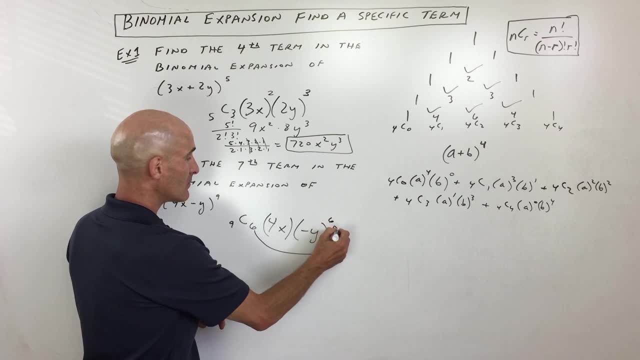 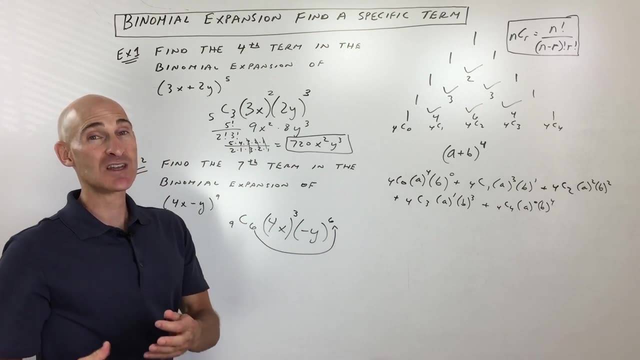 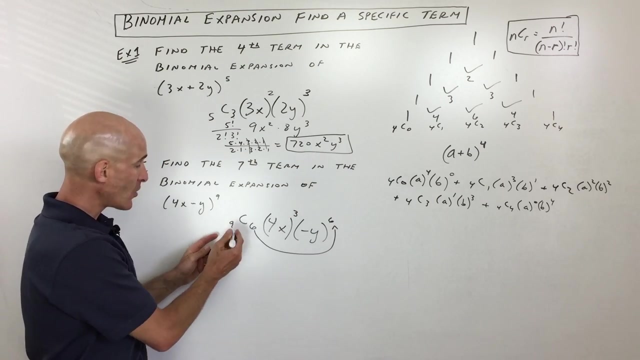 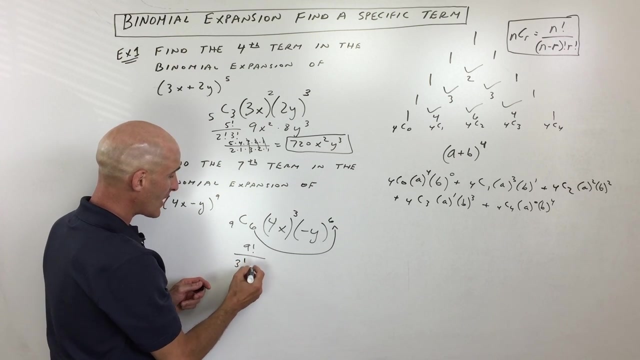 Remember this r value and this second term's power. those are always going to match and then these two powers are going to add up to nine. so this must be a three. So that's a quick way to get that particular term that you're looking for. Just remember it's the seventh term. It's actually going to be one less because you're starting at zero. So let's go ahead and simplify this now. So I'm using this combination formula: Nine choose six. This is actually nine factorial over nine minus six. three factorial times six factorial Four cubed is four times four times four. 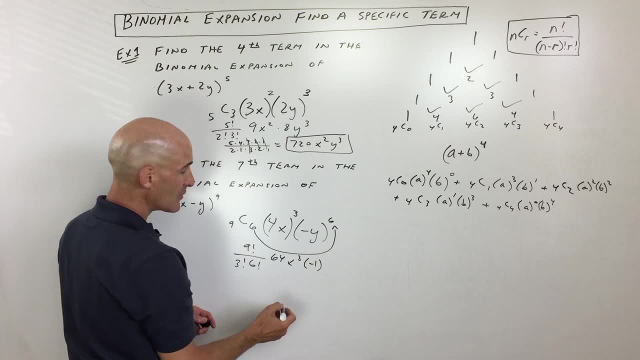 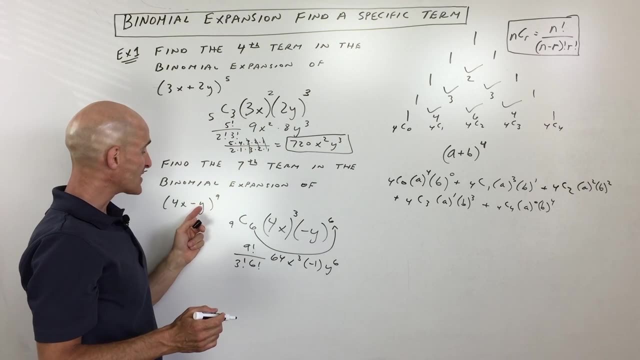 And then this is a negative one to the sixth power, which is going to be negative. one y to the sixth. Now notice, this one was plus. I didn't really put a plus here, but when it's a minus you can think of this as a negative one. so that's why I did negative one to the sixth power, which is just going to be negative, one to the sixth power, like that. Okay, so I'm just distributing. So now, if we simplify, what do we get? Well, we get nine factorial, which is nine times eight times seven times six, all the way down to one. Six factorial is six, five, four, three, two, one. 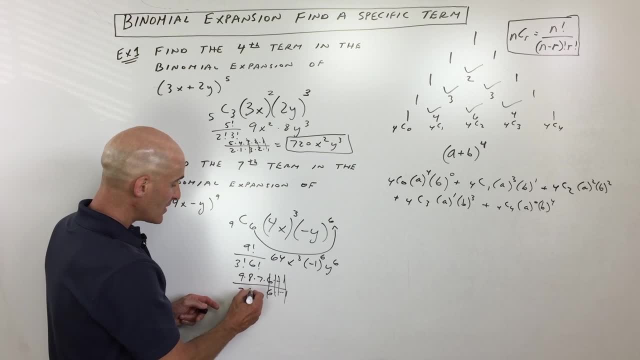 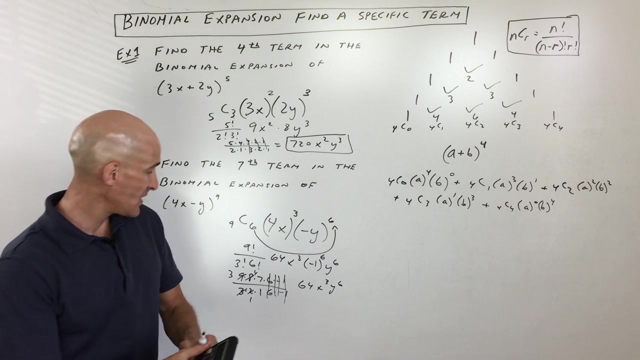 You can see those are canceling Three. factorial is three times two times one. Okay, and then here we have a negative one to an even, power is positive one. so that's going to be 64 x cubed y to the sixth. Things are shaping up here. Okay, let's see, We've got three goes into nine three times two, goes into eight, four times. So now we have 12 times seven, which is 84 times 64, right, So what's 84 times 64?? That's 5,376.